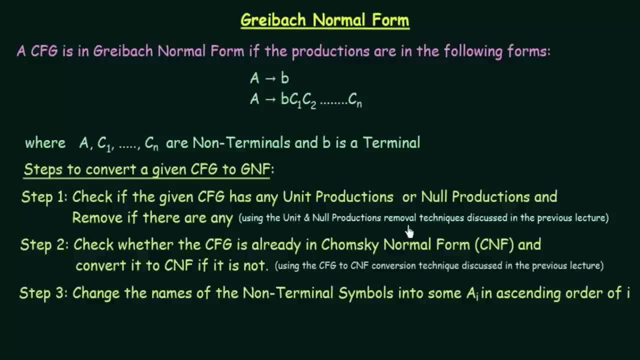 And also we have discussed how to remove the unit productions and null productions in one of the previous lectures, So you can watch that and, using that technique, you have to remove any unit productions or null productions that are present. Alright, so step number two. 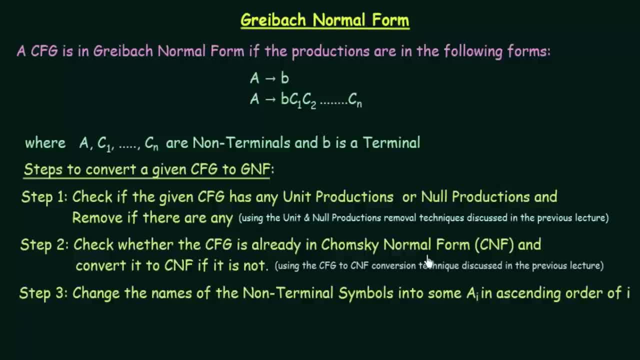 Check whether the CFG is already in Chomsky Normal Form and convert it to Chomsky Normal Form if it is not. So you have to check that the given CFG is it already in Chomsky Normal Form, And also you have to check that the CFG is it already in Chomsky Normal Form or not. 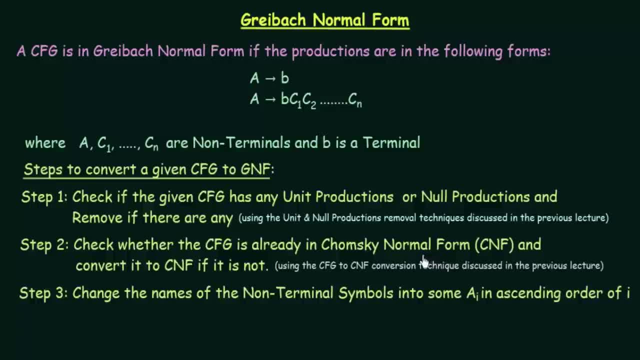 And if you don't know about Chomsky Normal Form, I advise you to watch the previous lecture, where we have discussed about Chomsky Normal Form And we have also discussed the steps that we need to follow in order to convert a given context-free grammar to Chomsky Normal Form. 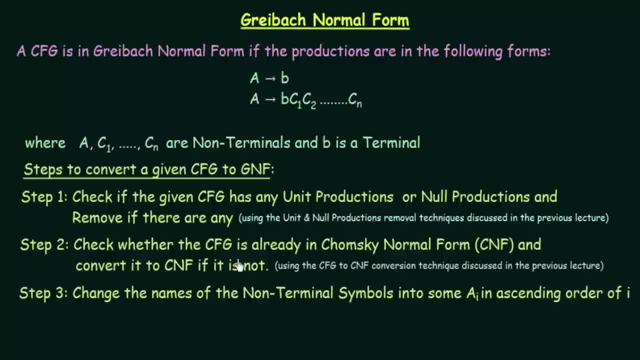 So in step two we have to check whether the given CFG is already in Chomsky Normal Form, And if it is not, you have to convert it using the technique that we have discussed in the previous lecture. And then step three says: 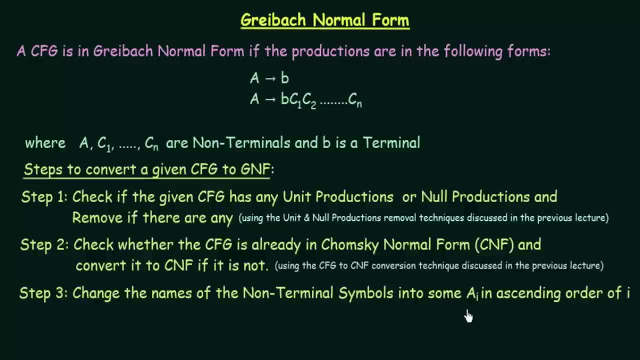 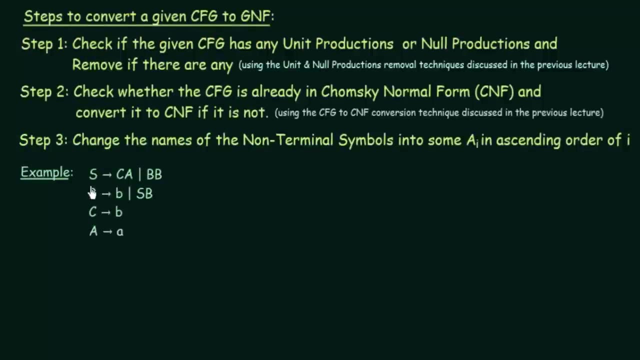 change the names of the non-terminal symbols into some errors of i in ascending order of i. now, what do we mean by this? we will see this using an example. all right, so here we have an example where we have a context-free grammar given and the productions. 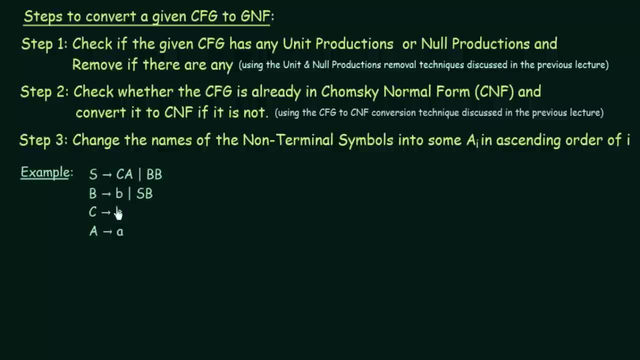 are of this form: s gives c, a and also b, b. b gives small b and also s b, c gives small b and a gives small a. so here the capital letters denote the non-terminal symbols and then the small letters they denote the terminal symbols. so let us just see step number one. we have to check if there are. 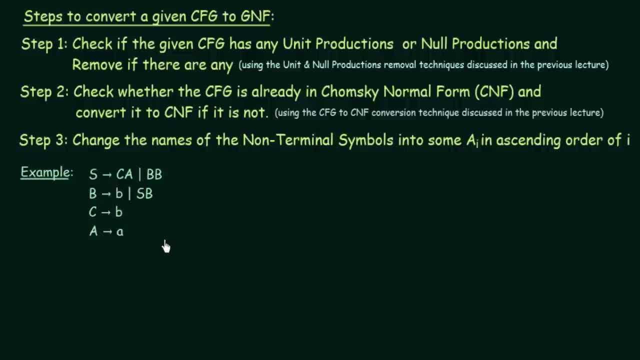 any unit productions or null productions. if you see that in these productions there are no unit productions or null productions, so step one, we don't have to do it. and step number two says: check whether it is already in chomsky normal form. so if you remember the rules that we need to follow, 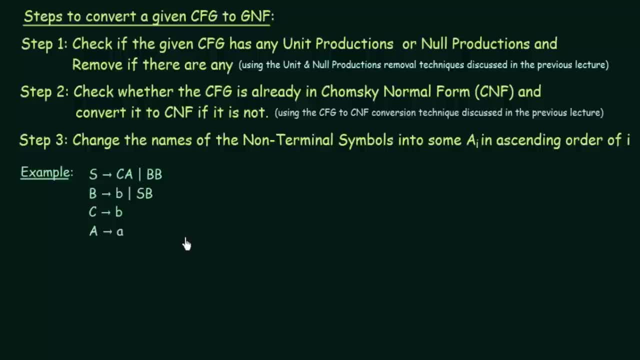 in order to check whether a given context-free grammar is in chomsky normal form and and using that, if we see, we see that this is already in chomsky normal form, you, so step two also is done. now step three says: change the names of the non-terminal symbols. 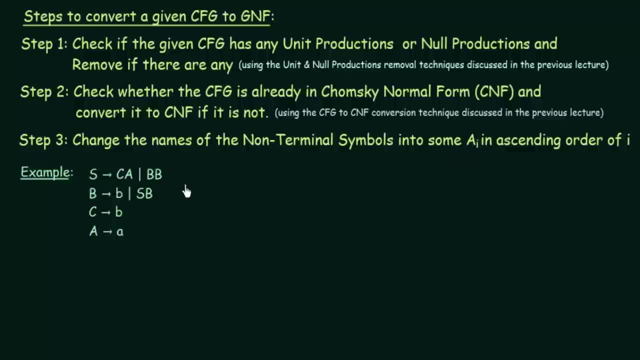 into some a of i in ascending order of i. now, how do we do this? for doing this, we see that we have the non-terminal symbols s, c, a, b in these productions and all this. we have to replace it with some a of i, and let's see how we can do this. so here we will replace s with a1 and then c with. 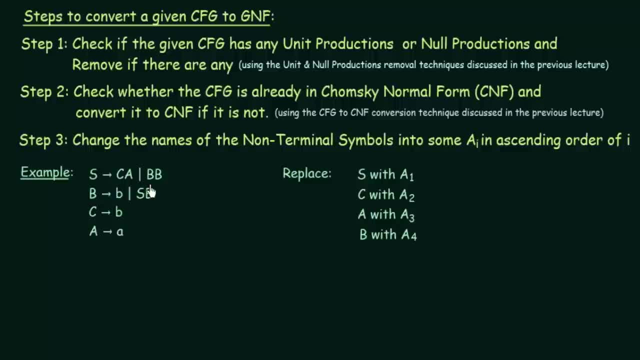 a1 and then a with a3 and b with a4. so this is how we will replace the names of this non-terminal symbols: using a of i where i is from one to four for this particular example. now you cannot just randomly give any names to these non-terminal symbols, but you have to follow it in ascending. 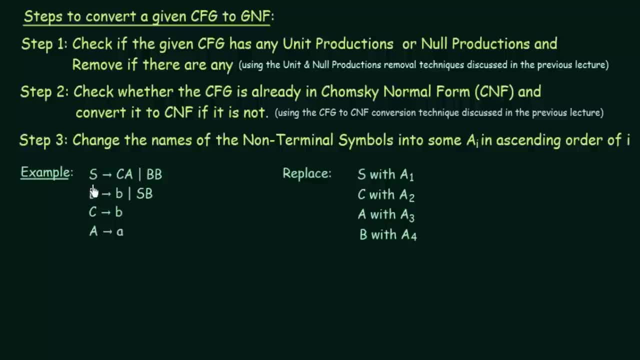 order starting from the very first production, so it's not that you just see s. okay, let me call it a of one. and then here i have b, so let me call it a of one and then a of d. so now we have b, so let me call it. 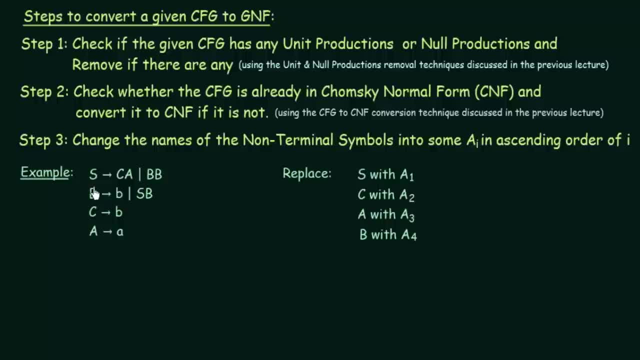 a of one, and then here i have b, so let me call it a of b. and then here i have b, so let me call it a of b, so A of 2, it's not like that. You have to first see the first production and you have to follow it in the correct order. 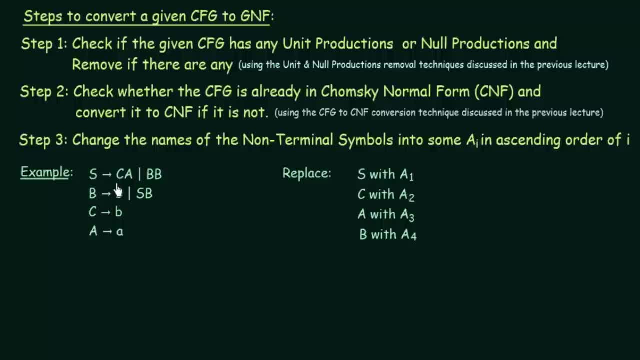 So here we have S, so I call it A of 1, and then the next one is C: I call it A of 2, A I call it A of 3 and B I call it A of 4.. 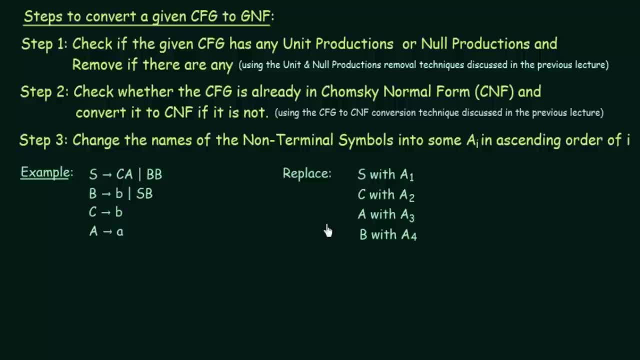 And if you come to the next production, it's B. we have already defined what is B and the next one is S- S also we have already given the name, and then C and A also we have already given. So we have to replace the variable like this: in ascending order: 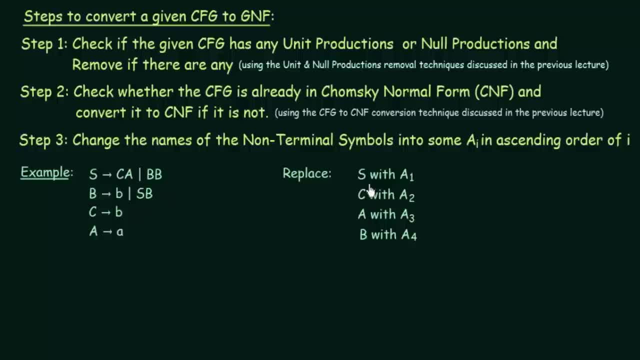 Now let's see what will be the equivalent production that we get after we replace these non-terminal symbols with these names: a1, a2, a3 and a4.. So this is what we get: A1 gives a2 and a3. 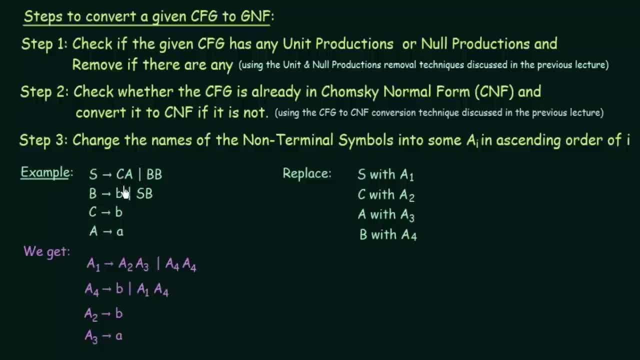 Did we get this? S was A1,. that is why I wrote here A1.. C was A2, that is why it is A2 and A was A3.. It's here, And so A1-C-C-A2 is A2 here and A was A3, that is why it is A3 and A4. 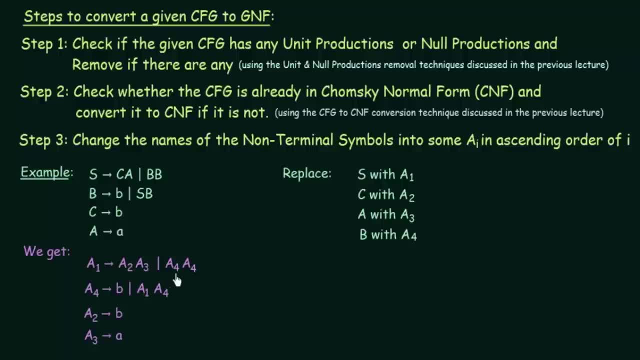 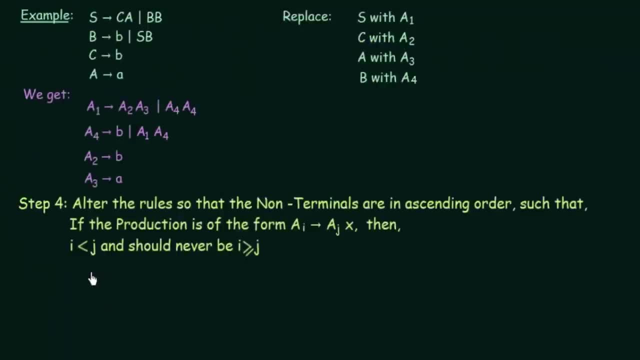 And so A1-C-C-C-A3 is a3-A2.. a3 here and both b's were a4. that's why you got a4, a4 here and the rest of the things also. when we replace it, this is what we get now let's see what is the next step, step number four. it says: 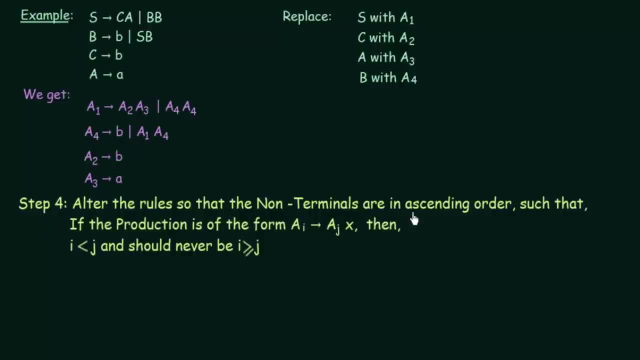 alter the rules so that the non-terminals are in ascending order, such that if the production is of the form a, i gives a, j, x, then i should always be less than j and it should never be greater than or equal to j. i should never be greater than or equal to j. so what do we mean by this? let us look. 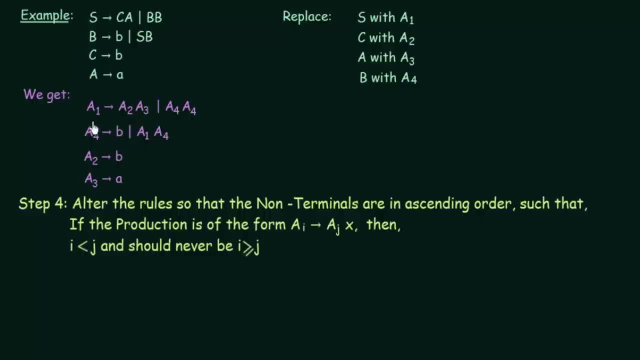 at this production. if you are taking this production, let's see and try to put it in the form of a i gives a j x. so here, what is our a i? it is a1, and what is our a j? it is a2 and you have. 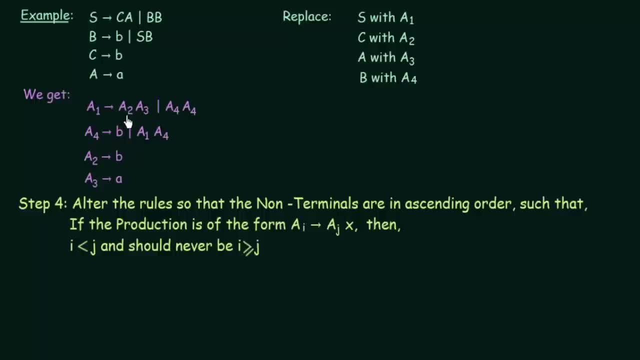 to just look at the first variable and the next one that follows it. you don't have to worry about the things after that. so here, your i is one you And your j is 2.. So our rule says that i should always be less than j. 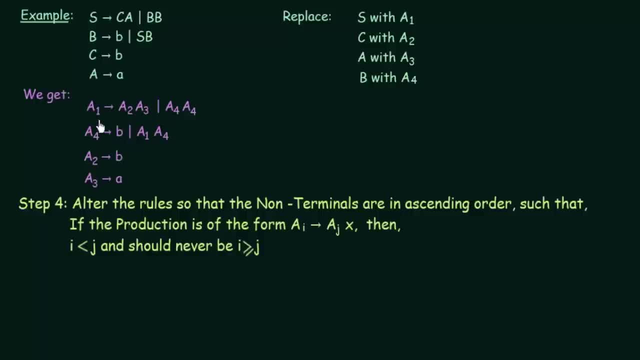 It should always be in ascending order, So let us see if it is the case here or not. So here i is 1 and j is 2.. i is definitely less than j. 1 is less than 2.. So it is following the rule which is mentioned over here. 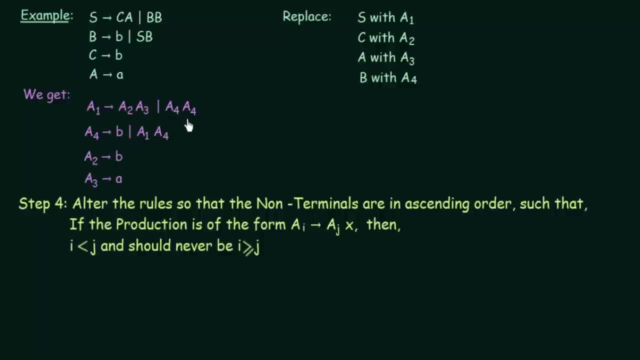 And let us see for the next one. a1 gives a4, a4. So you have to just look at a1 and this a4 over here. So here i is 1 and j is 4.. So 1 is less than 4.. 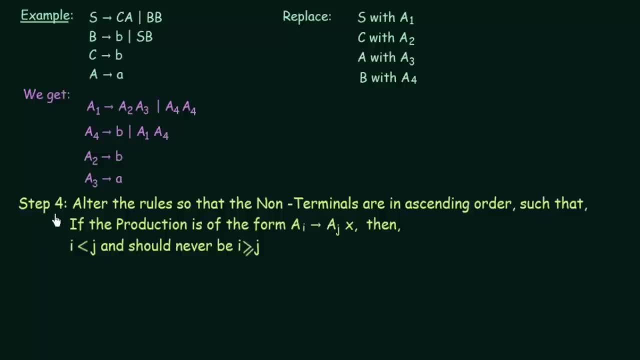 It is also in ascending order, So it is following the rule that is mentioned in step number 4.. So we are fine with this first production. And now let us check for the second production. Here it says a4 gives b. 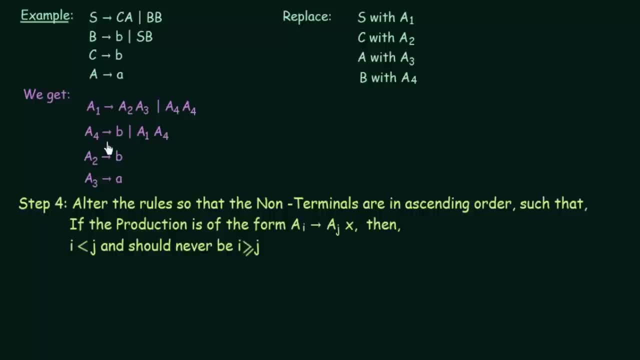 So what about this one? So when I already told you about the rules of Grebeck normal form in the beginning of this lecture, we saw that if a non-terminal symbol directly gives a terminal symbol, then that is already in Grebeck normal form. 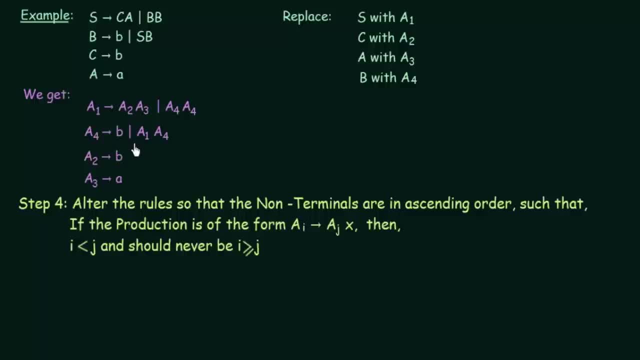 So this part is already in Grebeck normal form, You don't have to worry. So now we have to look at this part. So in this part it says a4 gives a1, a4. Now let us see if it is following step number 4 or not. 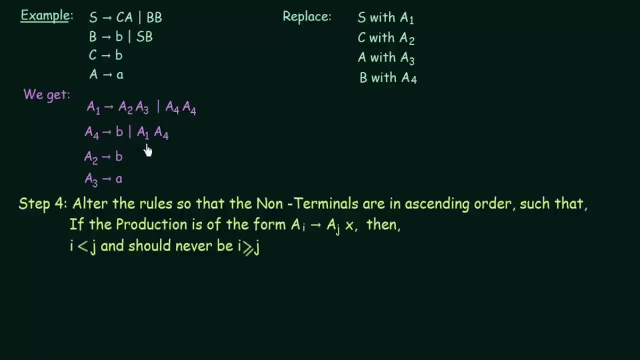 So here, your i is 4 and j is 1.. So here we see that i is greater than j, 4 is greater than 1.. So we already said in step number 4, the rule said that it should never be greater than or equal to j. 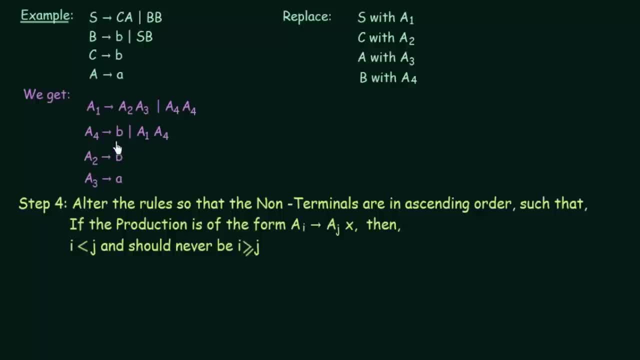 It is not following the rule that is mentioned in step number 4.. So we need to resolve this portion. Now let us see how we can resolve it. We have to resolve it by replacing the problematic variable with some other values. So let us see how we can do that. 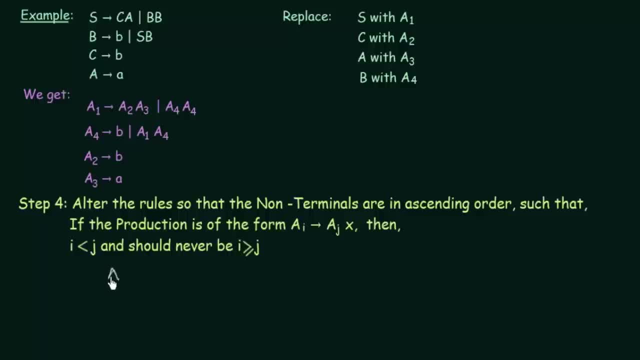 So here let me just write down the rule that is causing the problem. It is: a4 gives b, a1 gives a1.. Now, if you look at this, the problem is caused by this a1 over here. So what I will do is I will replace this a1 with some other value. 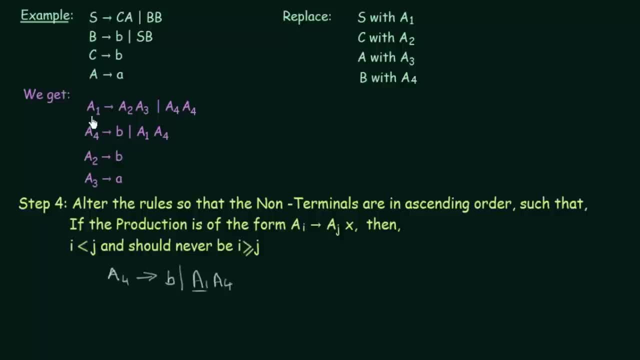 Now, what is that? some other value with which I can replace a1?? I have to replace it with the value of a1 that is given over here. So let us replace it and see if it is going to follow the rule or not. 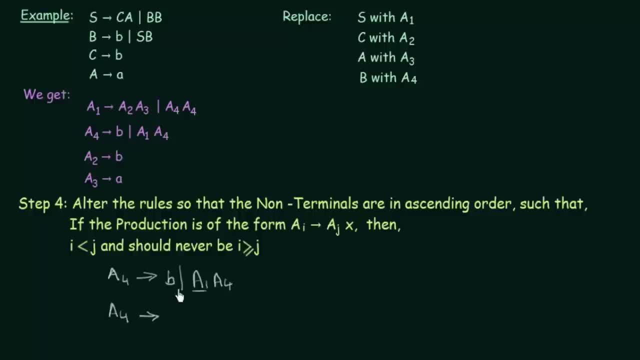 So I will write a4. it gives now this b. I will write it as it is, and then instead of a1, I will write a2, a3 and a4, a4.. So first let me write this one: a2, a3. 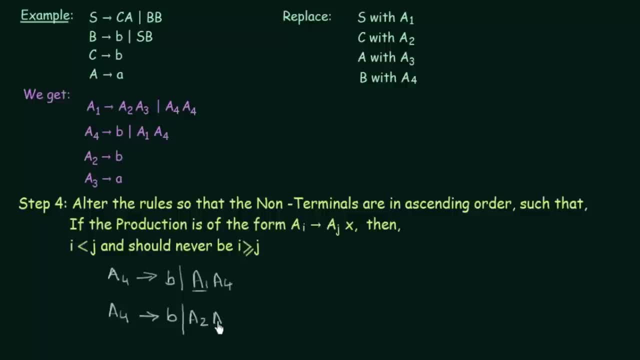 So I will write a2, a3 and this a4 which is here, I have to write it down as it is a4 and also it gives a4, a4.. So instead of this a1, I will put a4, a4. 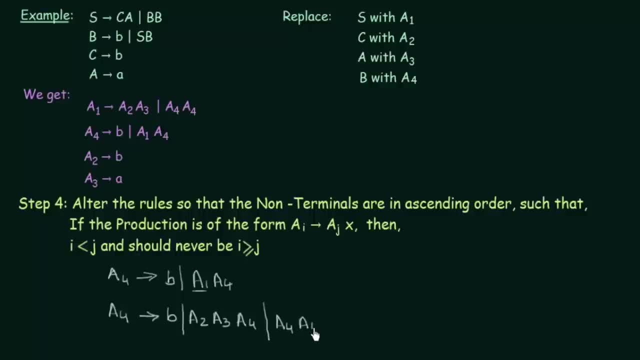 a4, a4 and this a4 which is here- I will write it down as it is- a4- Alright, so now we have this production. Now let us see if it is following the rules that was mentioned in step 4 or not. 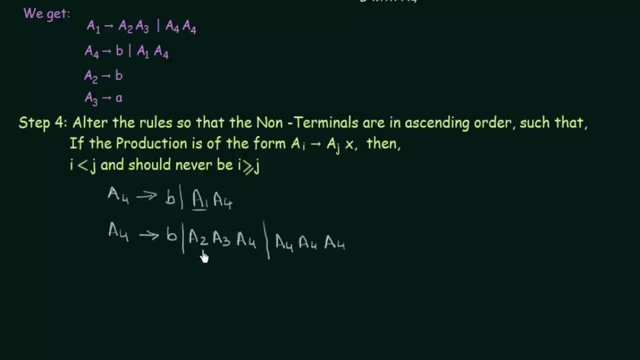 a4 gives b. that is fine. Now a4 gives a2, a3, a4.. Now let us check here. our i is 4 and our j is 2.. Again, we see that i, which is 4, is greater than j, which is 2.. 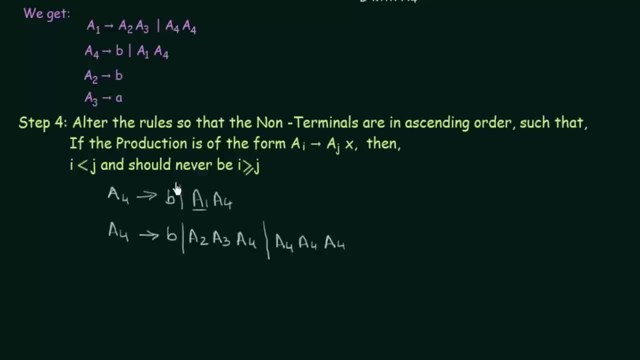 So this is not allowed. So it is still not following the rule of step number 4.. So what I will do is I will replace the balance. I will replace the value of a2, because this was the variable that is causing the problem. 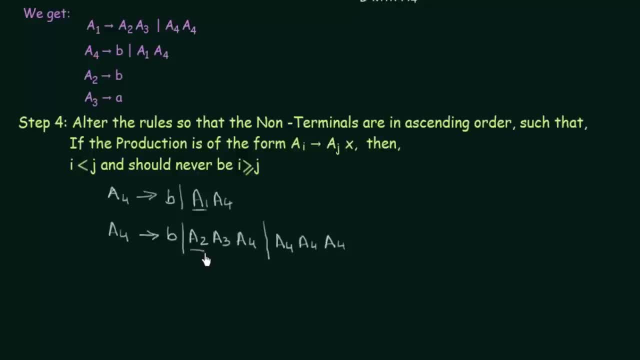 I will replace the value of a2 with some other value in order to make it follow rule number 4.. So what is the value of a2 with which I can replace it? a2 gives b. Now let me try to replace a2 with b. 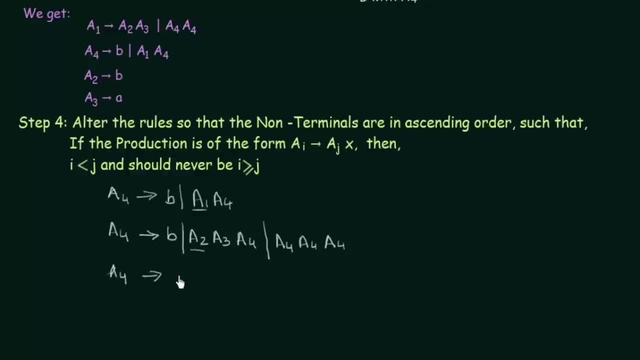 So this a4, let me write it a4, it gives b, This b as it is, And instead of a2, I will write b, now b and the rest of the things I will write as it is: a3,, a4 and this part also, I will write it as it is. 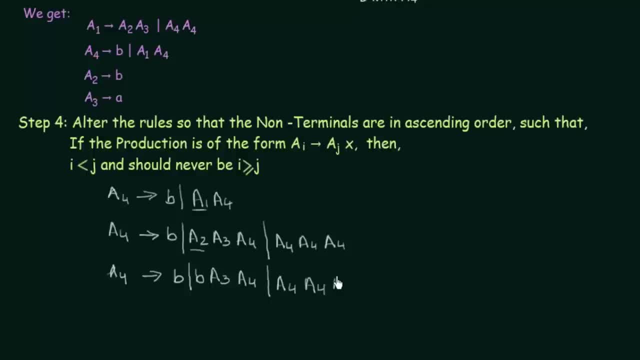 a4, a4, a4.. Now let us see if it is following our rules or not. So here we see that a4 gives b- Okay, that is fine, And a4 gives b, a3, a4.. 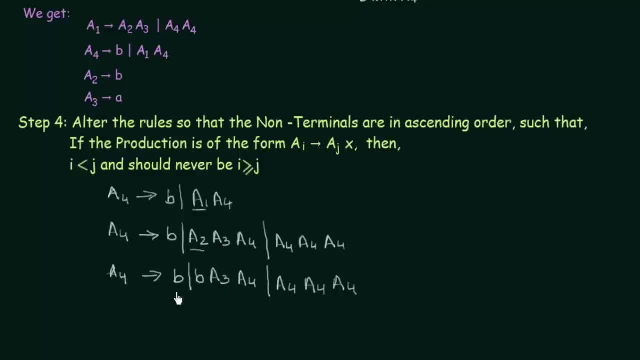 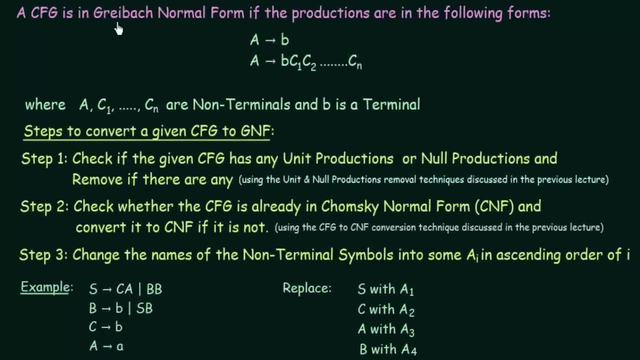 Now, if you remember the rules of GRIBAC Normal Form, if a non-terminal symbol gives a terminal symbol followed by anything, then that is in GRIBAC Normal Form. So let me just take you up there once. So if you see here a CFG is in GRIBAC Normal Form. 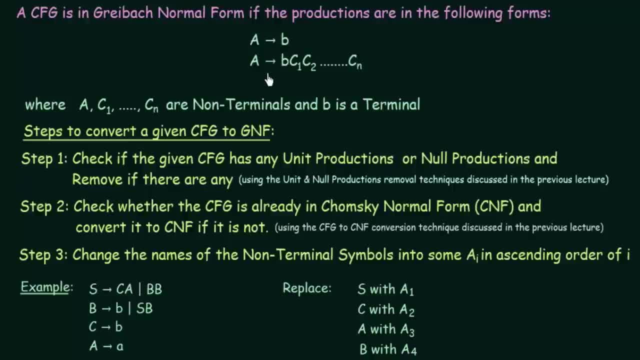 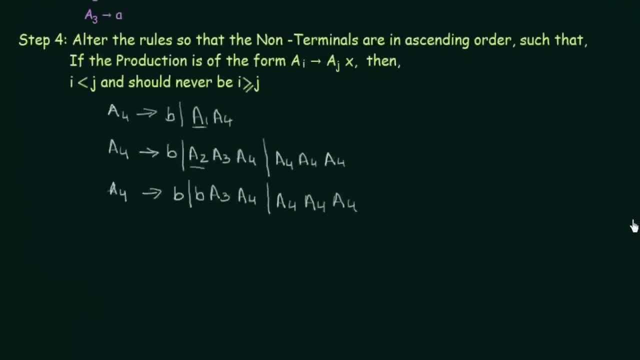 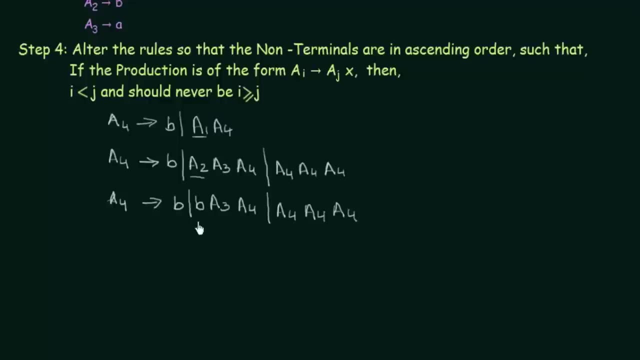 if it is giving a terminal symbol directly, or if it gives a terminal symbol followed by any other variables, then also it is in GRIBAC Normal Form. So we see that this part is in GRIBAC Normal Form. now b and b, a3, a4 are already in GRIBAC Normal Form. 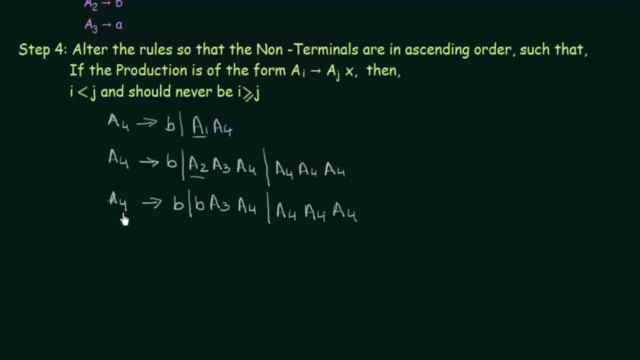 Now we have to check this part. It says a4 gives a4,, a4, a4.. Here our i is 4 and j is also 4.. So here we are getting a condition, a situation where i is equal to j. 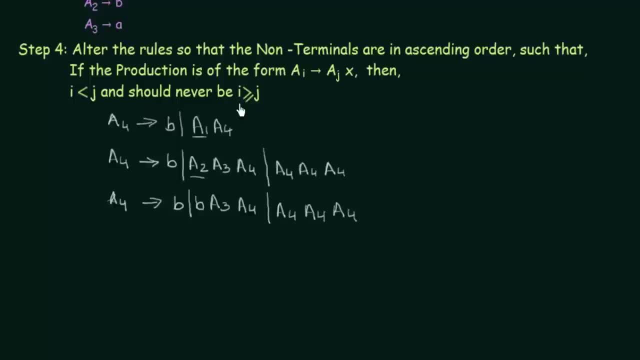 So that is also not allowed In step 4, it says it should never be- i is greater than or equal to j. So here we are getting a condition where i and j are equal. So when we get this, what we have to do